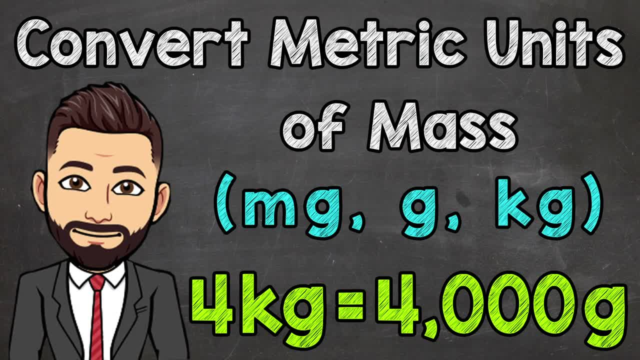 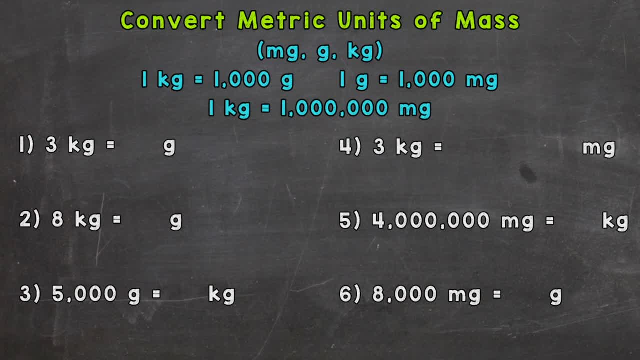 Welcome to math with Mr J. In this video we're going to be converting metric units of mass, and specifically milligrams, grams and kilograms, and our base unit of mass for the metric system is going to be a gram, so everything's going to be based around that gram and the other units of 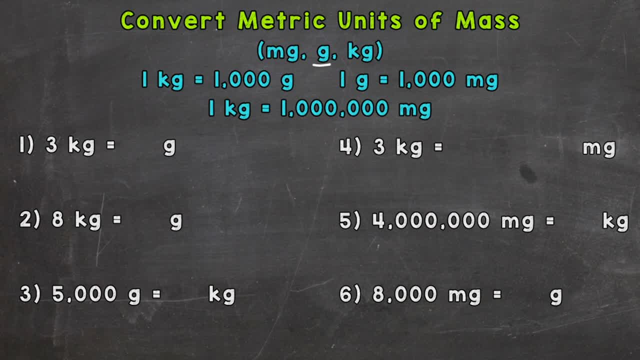 mass are going to have prefixes attached to gram and that's going to tell us what those units of mass mean. so for example, milligram, the prefix milli means 1, 1,000. so a milligram is one one thousandth of a gram. therefore a thousand milligrams equals one gram. and for a point. 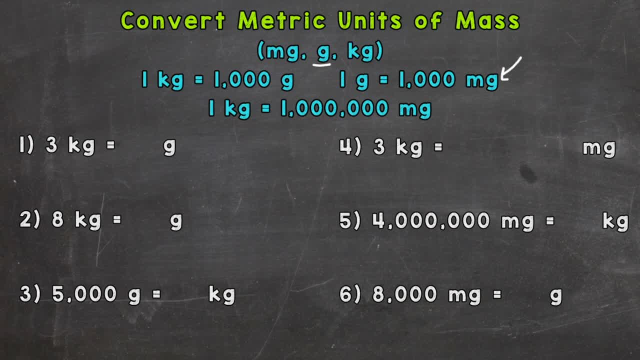 of reference, a milligram is one thousandth of a gram is a unit of mass. that is about a grain of salt or sand. Next we talked about our base unit, gram, and for point of reference, a gram is about a paperclip or stick of gum. 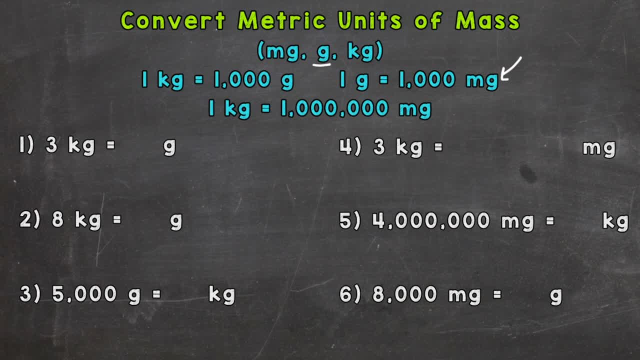 And then kilogram. we have the prefix kilo. that means 1,000. So it takes 1,000 grams to equal one kilogram, And a kilogram is a little over two pounds. so about the mass of a textbook? 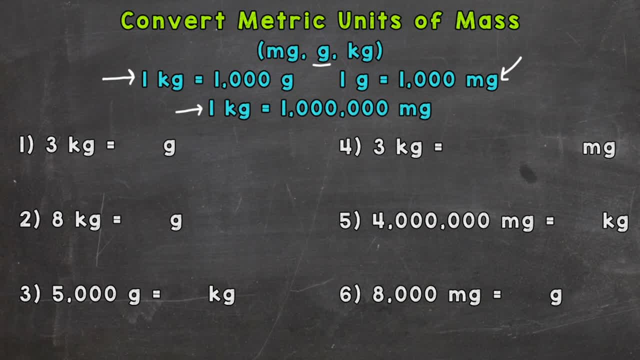 And then down here we have one last note: one kilogram equals a million milligrams. So let's jump into some conversions here, where we're going to convert between milligrams, grams and kilograms. So number one: three kilograms equals how many grams? 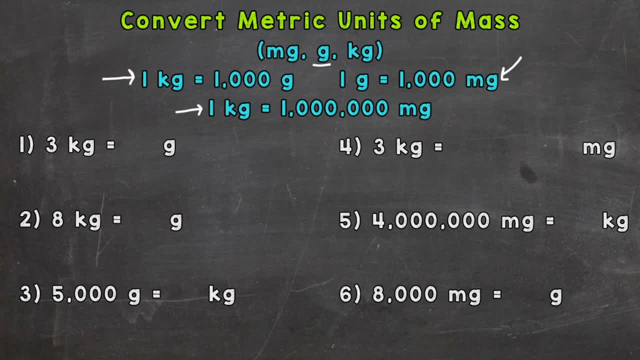 Well, one kilogram equals 1,000 grams, but we have three, so 1,000, 1,000, 1,000.. So we can do three times 1,000 to give us how many grams that would equal. 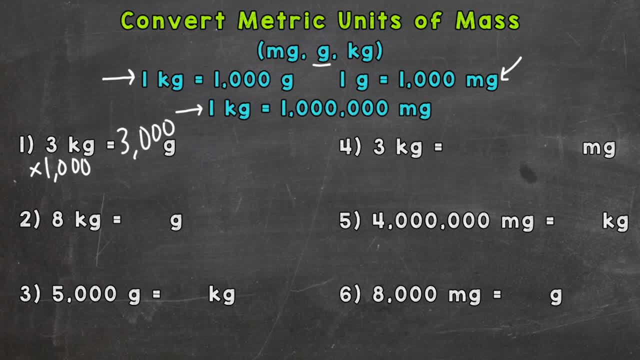 And that's going to give us 3,000 grams. Next we have eight kilograms. equals how many grams? So eight groups of 1,000, 1,000, 1,000, 1,000, 8,000.. 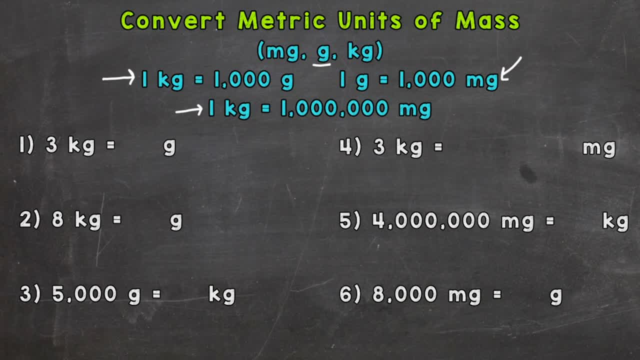 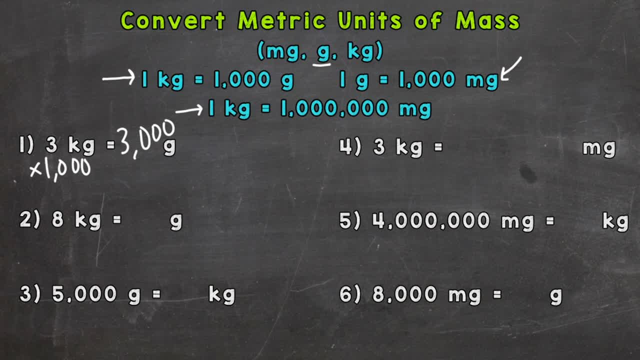 8 groups of a thousand times. So when we're going from kilograms to grams, we multiply by a thousand, Just like number one, except we have eight kilograms here. So we're going to end up with eight thousand grams. Eight kilograms equals eight thousand grams. 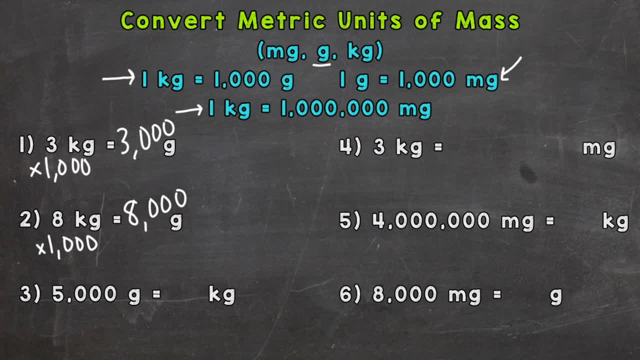 For number three, we're going to go the opposite way. We're going to go from grams to kilograms. So we start with five thousand grams and we need to split that five thousand into groups of a thousand, Each one of those groups of a thousand. 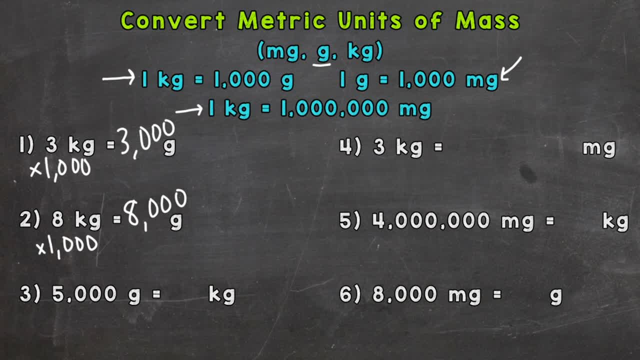 equals one kilogram. So when we're going from grams to kilograms, we need to divide by one thousand. Five thousand divided by a thousand equals five. you number four. we're going from kilograms to milligrams, so three kilograms. each one of those kilograms is a million milligrams, so a million, a million, a million, so we do three. 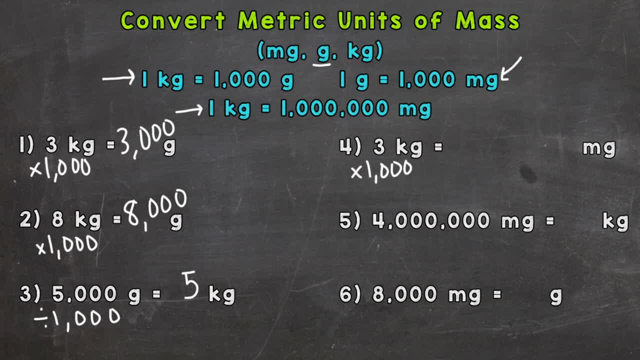 times a million, and that's going to give us an answer of three million milligrams number five. we're going the opposite way. so we're going from milligrams to kilograms, so we need to split into groups of a million. each one of those millions is a kilogram, so we need to do four. 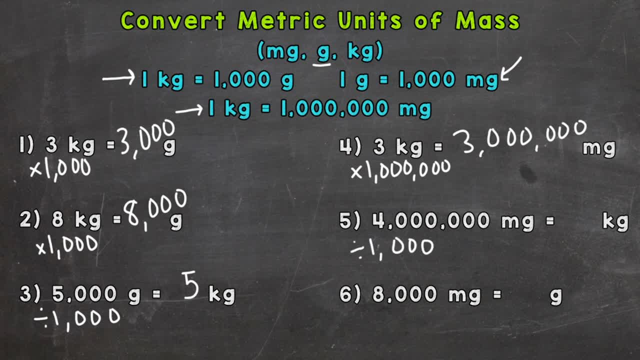 million divided by a million, and we end up with four kilograms. so four million milligrams equals four kilograms. and lastly, number six: eight thousand milligrams equals how many grams? well, we need to split into groups of a thousand. each one of those a thousand is a one. 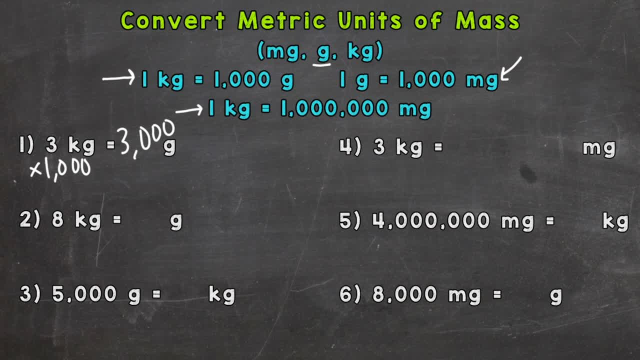 Eight times. So when we're going from kilograms to grams, we multiply by 1,000, just like number one, except we have eight kilograms here. So we're going to end up with 8,000 grams. Eight kilograms equals 8,000 grams. 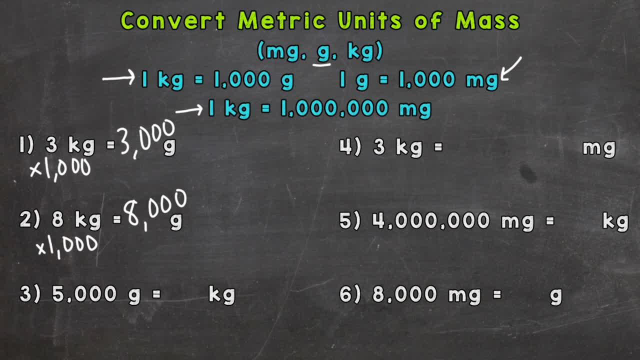 For number three, we're going to go the opposite way. We're going to go from grams to kilograms. So we start with 5,000 grams. So we start with 5,000 grams. So we start with 5,000 grams. 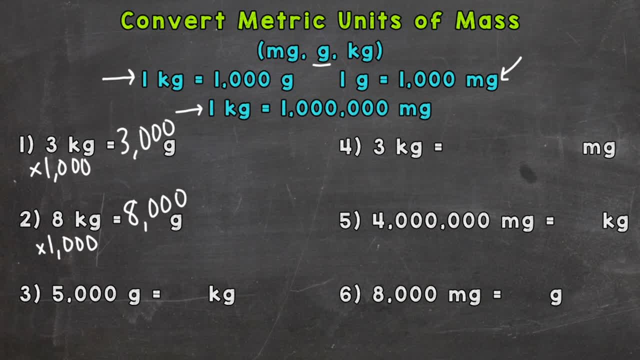 And we need to split that 5,000 into groups of 1,000.. Each one of those groups of 1,000 equals one kilogram. So when we're going from grams to kilograms, we need to divide by 1,000.. 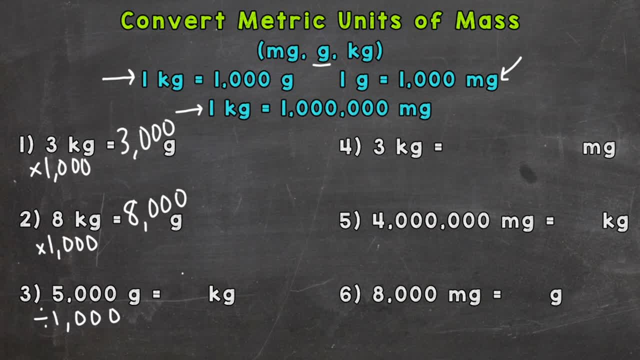 5,000 divided by 1,000 equals five. Number four: we're going from kilograms to kilograms. Number four: we're going from kilograms to milligrams. So three kilograms. Each one of those kilograms is a million milligrams. 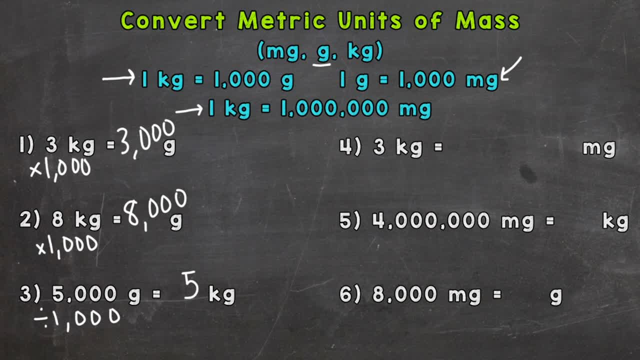 So a million, a million, a million, So we do three times a million And that's going to give us an answer of three million milligrams. Number five: we're going the opposite way, So we're going from milligrams to kilograms. 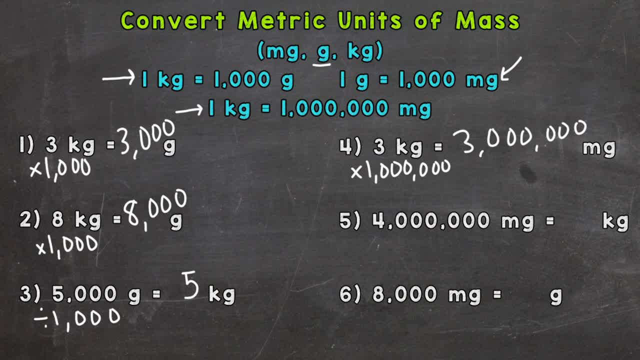 So we need to split into groups of a million. Each one of those millions is a kilogram, So we need to do four million divided by a million And we end up with four kilograms. So four million milligrams equals four kilograms. And lastly, number six: 8,000 milligrams equals how many grams? 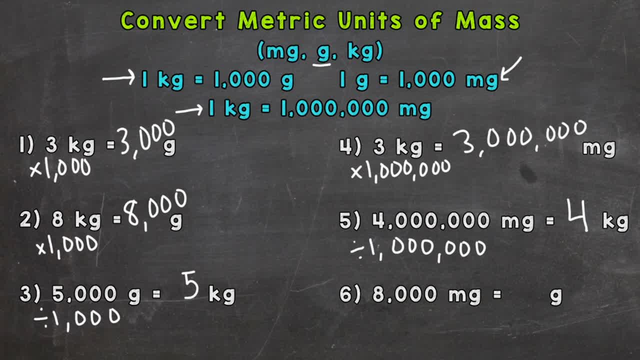 Well, we need to split into groups of 1,000.. Each one of those 1,000 is a one gram. So milligrams to grams divide by 1,000. And we end up with eight grams. So there you have it. 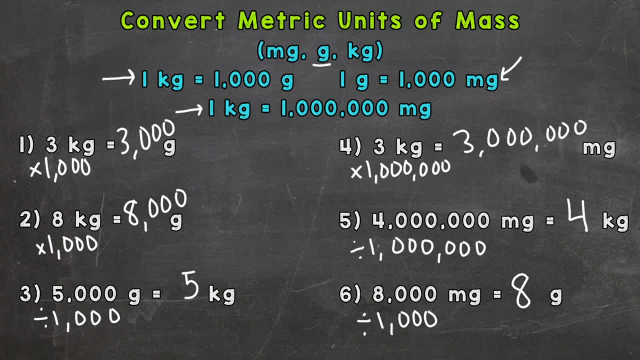 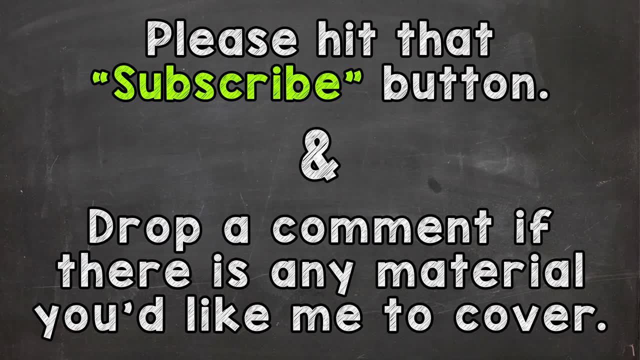 There's converting metric units of mass with milligrams, grams and kilograms. Hopefully you found this helpful. Hopefully that helped. Thanks so much for watching. Until next time, peace.